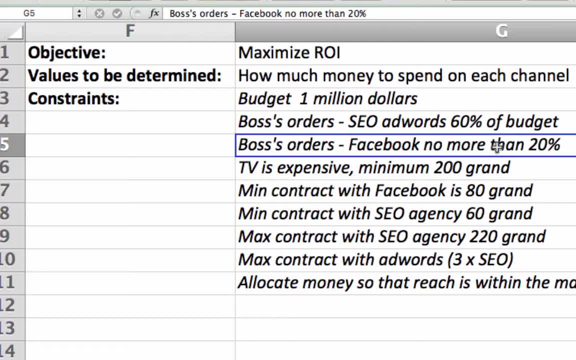 you can't spend more than $200,000.. You know TV is expensive. There's lots of production costs associated with it. It's going to be at minimum 200 grand and you need to take that into account. You know that the minimum contract with the Facebook agency is 80 grand. 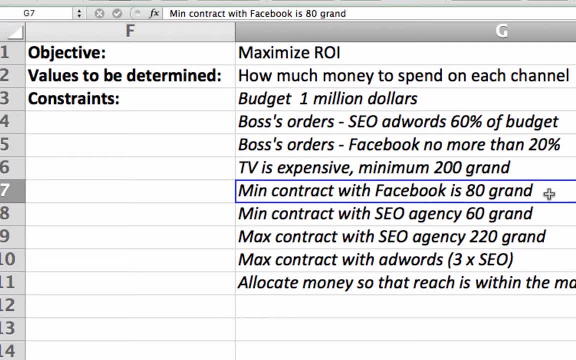 They don't even listen to clients who aren't going to spend that much. The minimum contract with the SEO agency is 60 grand and they also have a maximum. the SEO agency doesn't want to. they don't do accounts greater than 220 grand because they don't have the resources for that and we sort of had a 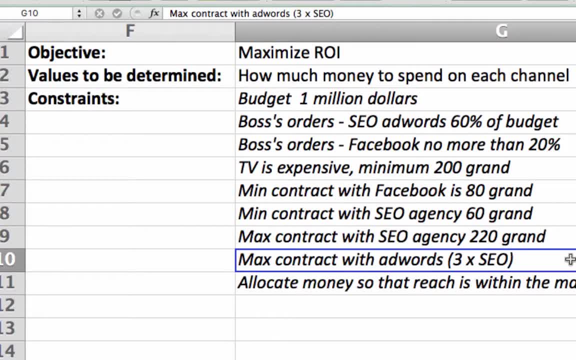 piece of imaginary wisdom handed down to us from the SEO experts that the maximum contract: you shouldn't spend more than three times of your SEO budget on AdWords. so whatever we spend on AdWords needs to be, you know, less than three times what we spend on SEO. now there's another, more interesting another. 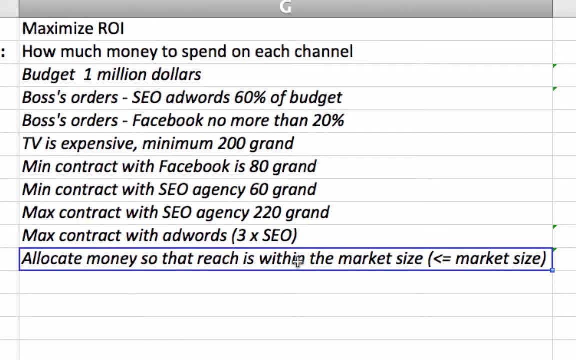 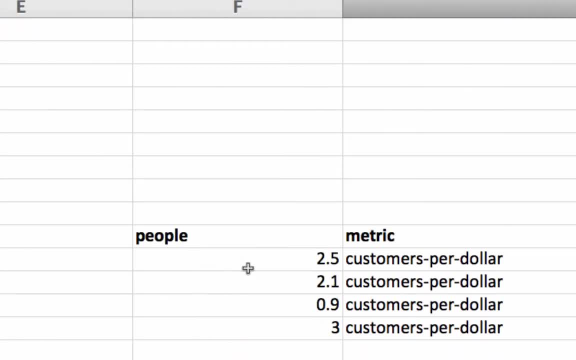 interesting constraint, which is we want to allocate our money such that our reach is within the size of our market. now the size of our market is 1.3 million, so you can see that number represented, represented down here. we've got a market size that much it doesn't really make sense to 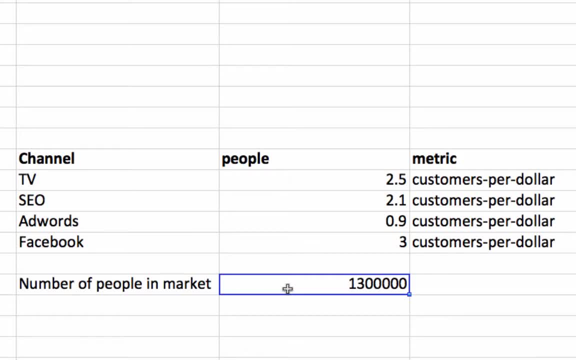 advertise I outside that market And we also have these sort of spread or reach metrics that were handed down to us as well, which that described these outlets- TV, SEO, AdWords and Facebook- And we know that within each one- so for example, in TV, we get 2.5 customers per dollar, SEO, 2.1 customers per. 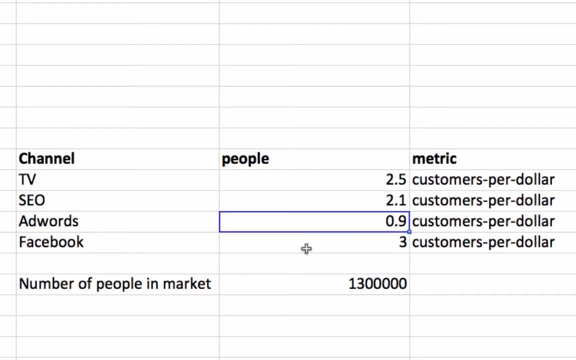 dollar. AdWords 0.9 customers per dollar and Facebook we get three customers per dollar. So this is sort of a complicated situation we're in here. We have these estimates of reach, we have these estimates of the proportion ROI per channel and we have all these constraints. 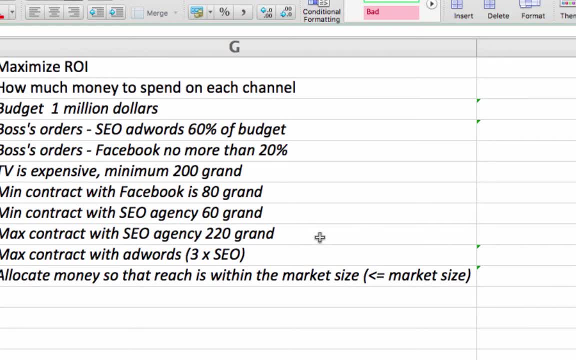 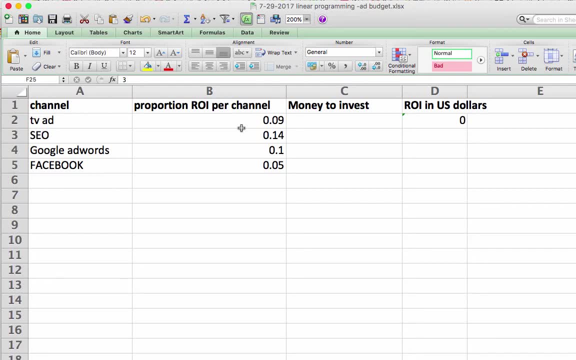 that we've been given. So how do we figure out how much money we should spend in each one of these channels? This is a classic linear programming problem. In linear programming you need to have three things. So any problem in business, or really any problem if you can break.